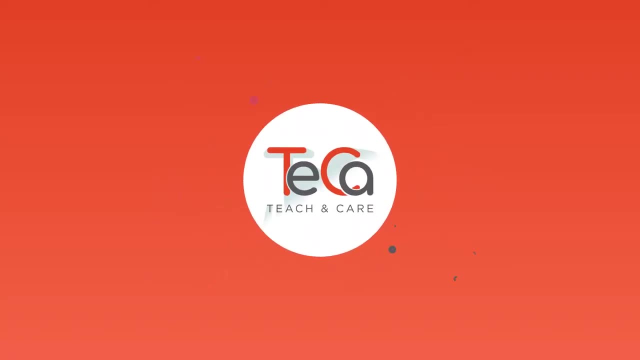 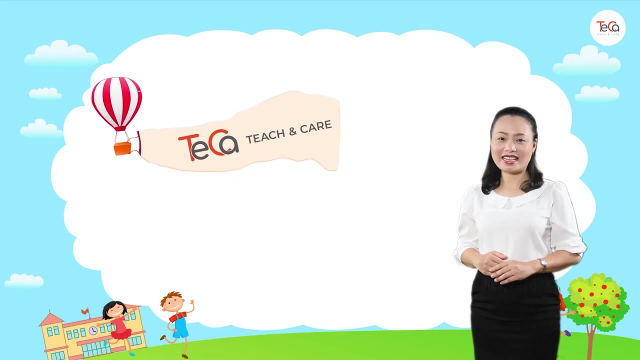 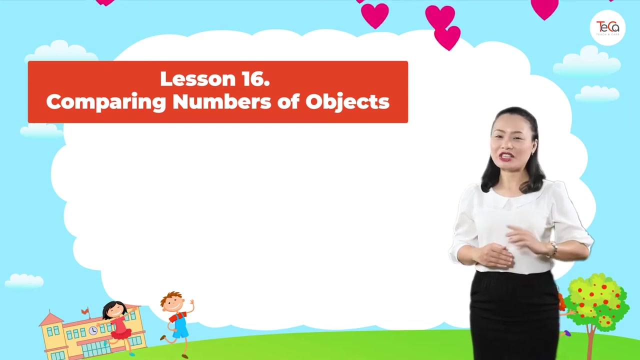 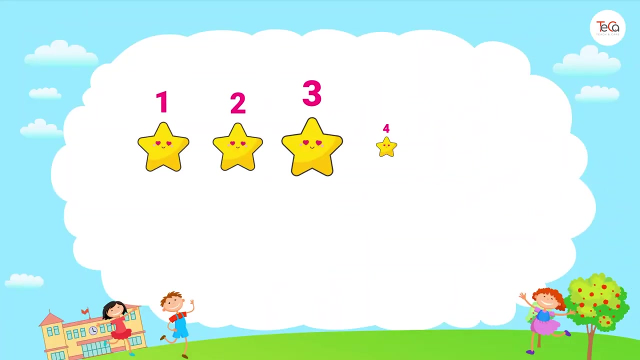 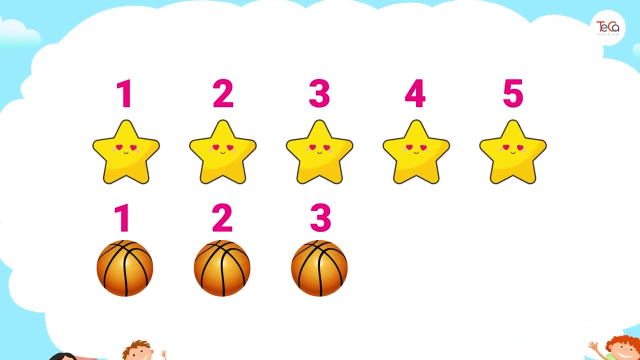 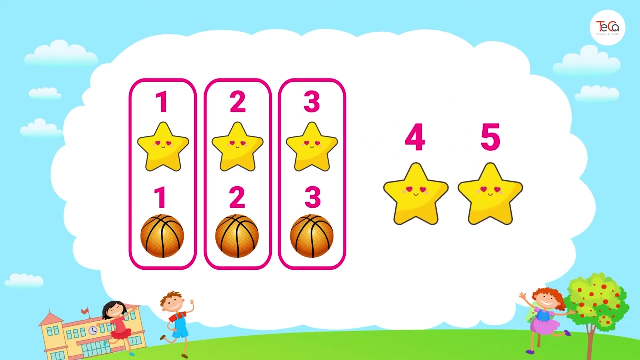 Hello children, In this lesson we're learning to compare numbers of objects. Stay tuned. Look, we have five stars and three balls. If we pair a star with a ball, then two stars are unpaired, because there are more stars than balls. 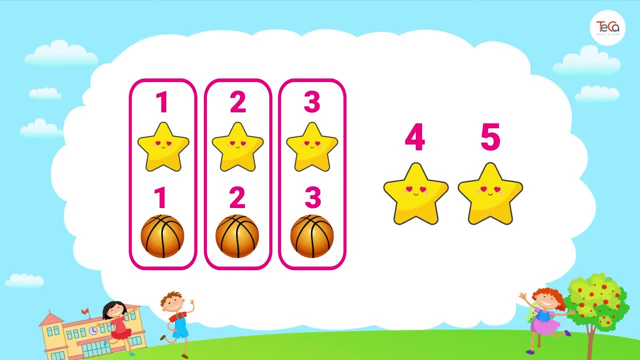 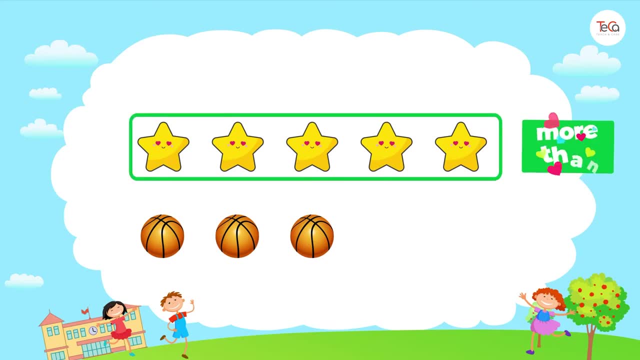 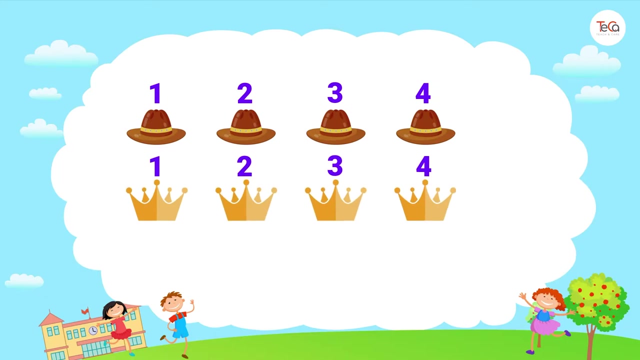 Or there are fewer balls than stars. So we say the number of stars is more than the number of balls, Or the number of balls is less than the number of stars. Next, we have four hats and four crowns. If we pair a hat with a crown, then two stars are unpaired because there are more stars than balls. 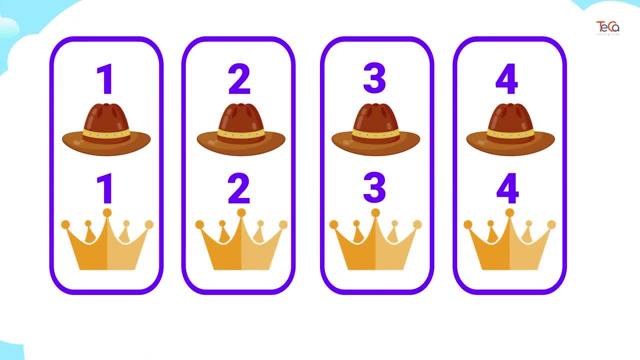 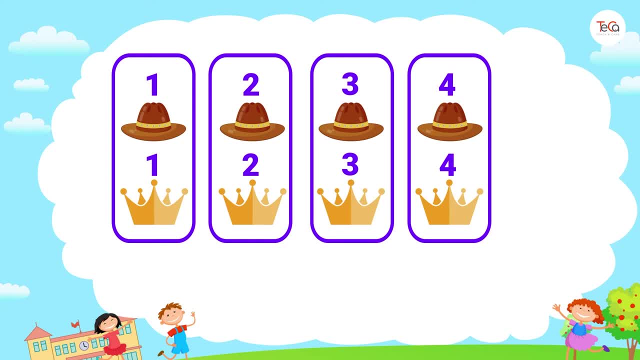 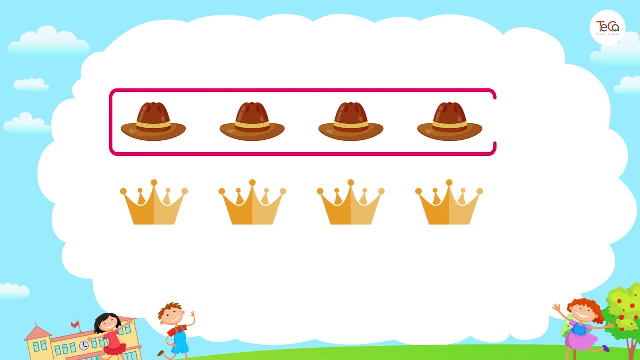 Or if we pair a hat with a crown, then each hat is paired with a crown because there is an equal number of hats and crowns. So we say the number of hats is equal to the number of crowns, Or the number of crowns is equal to the number of hats. 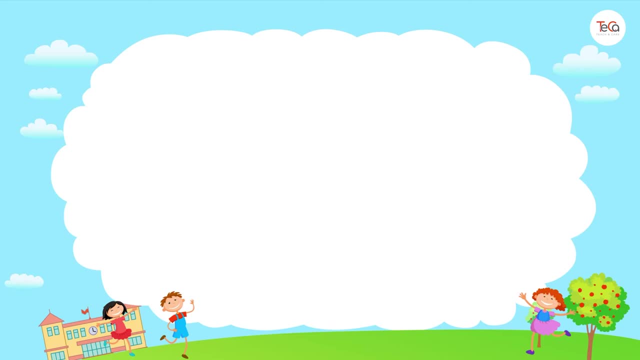 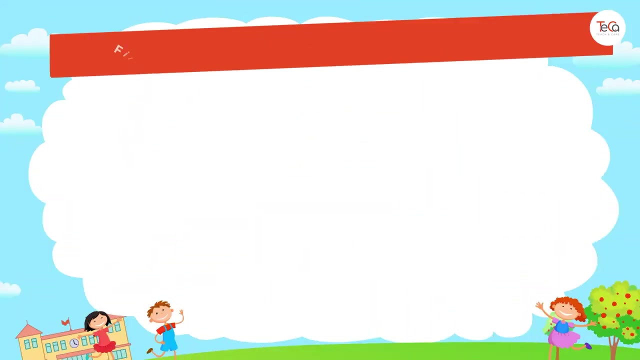 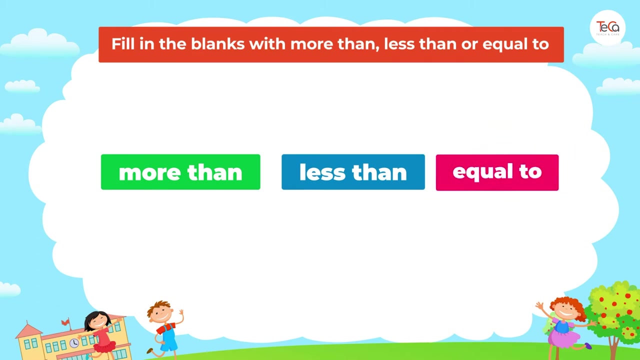 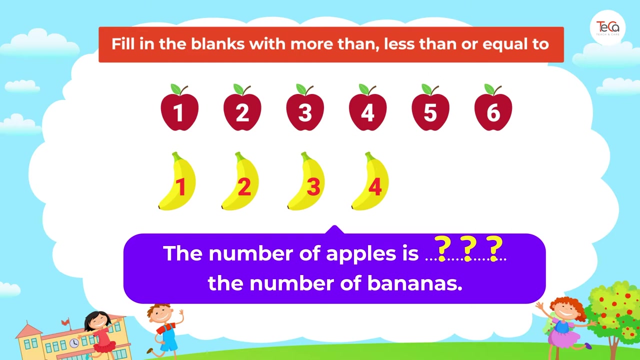 I hope you understand More than, less than and equal to. Now let's get some practice. Fill in the blanks with more than, less than or equal to. Look here: we have six apples and four bananas. The number of apples is the number of bananas. 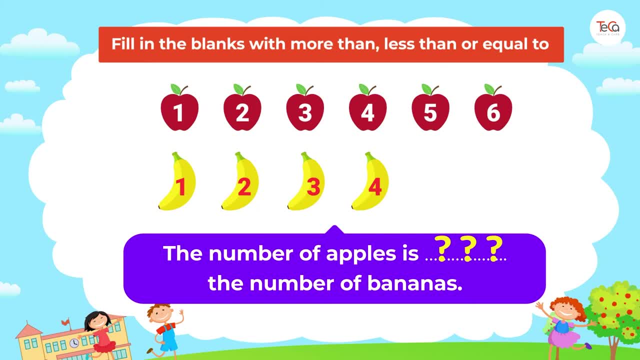 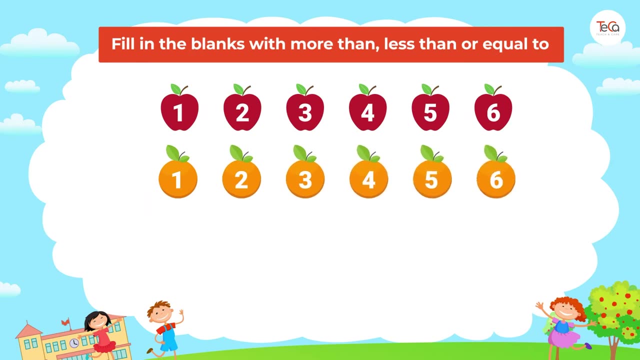 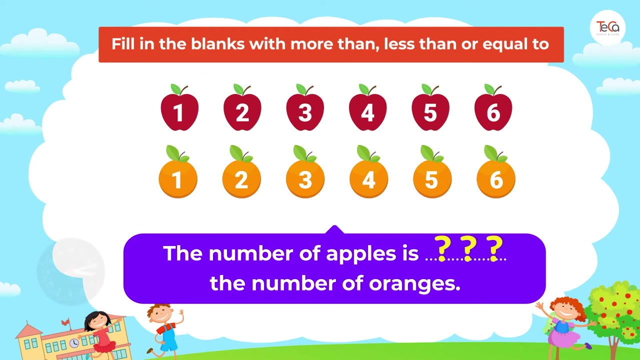 Have you got your answer? So the number of apples is more than the number of bananas. Next, we have six oranges. The number of apples is more than the number of bananas. The number of apples is the number of oranges, So the number of apples is equal to the number of oranges. 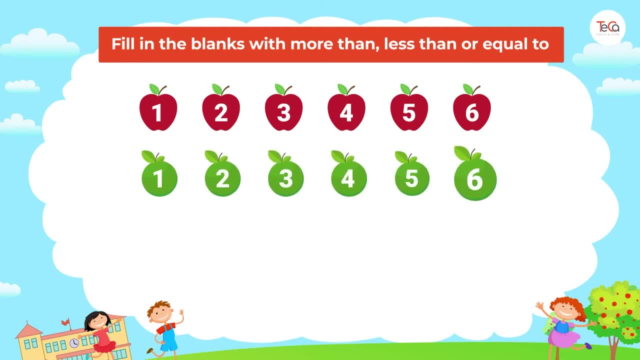 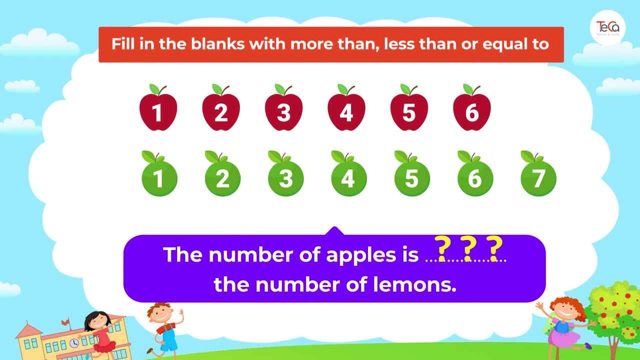 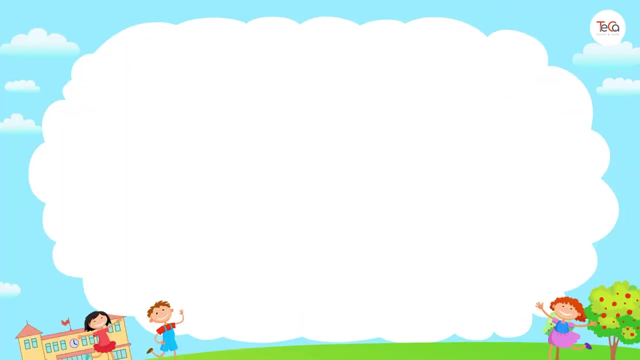 Next we have seven lemons. The number of apples is the number of lemons. The number of apples is less than the number of lemons, So the number of apples is less than number of lemons. Now we have a number of bees and butterflies. 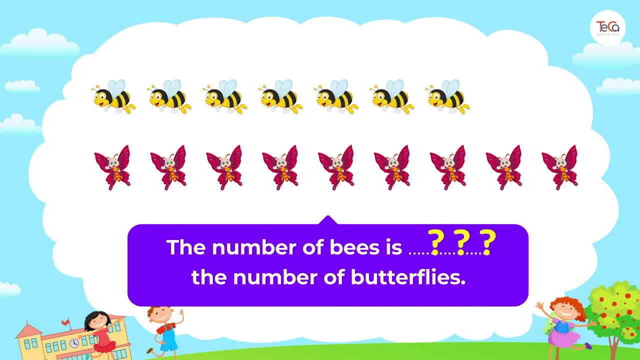 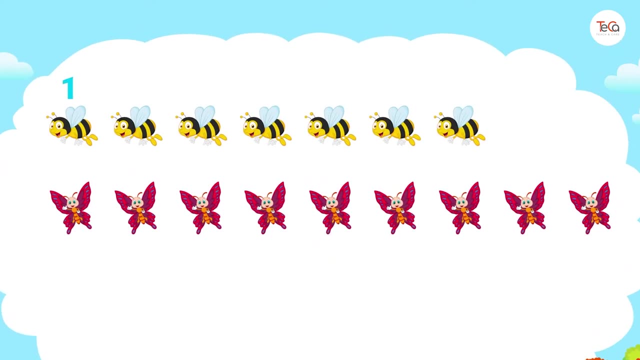 The number of bees is the number of butterflies. Systems, Systems, Systems, allergies, Diabetes, Diabetes. Do you have your answer yet? First, let's count the number of bees: 1,, 2,, 3,, 4,, 5,, 6,, 7.. 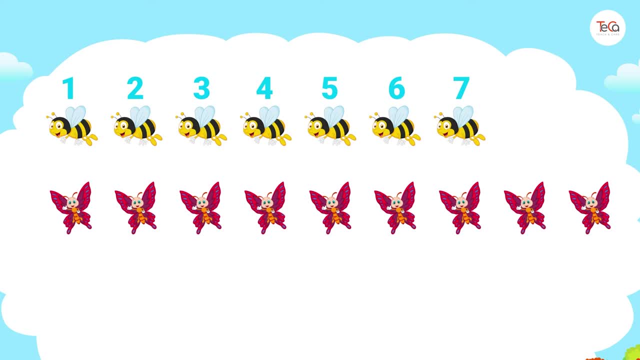 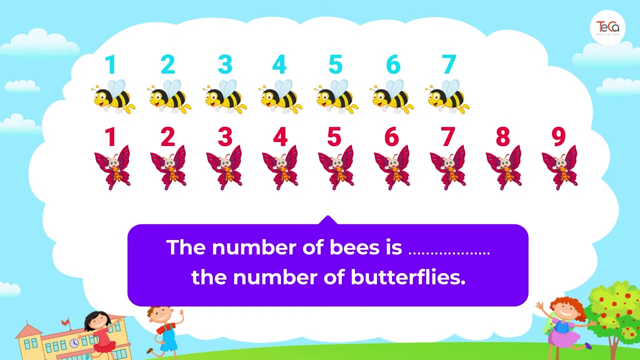 Now let's count the number of butterflies: 1,, 2,, 3,, 4,, 5,, 6,, 7,, 8,, 9.. So the number of bees is less than the number of butterflies. 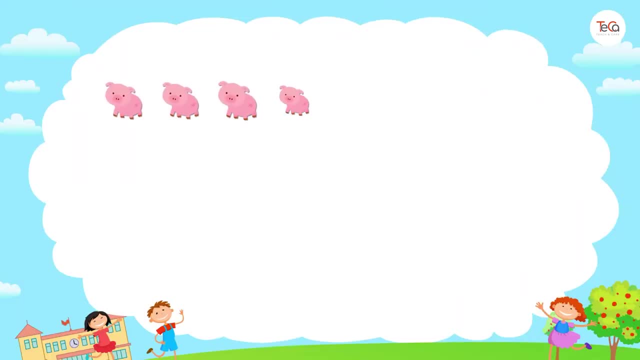 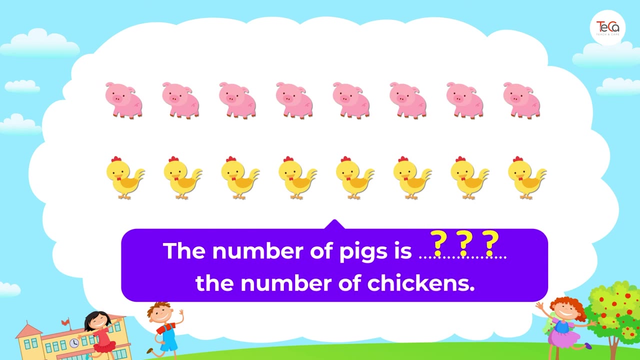 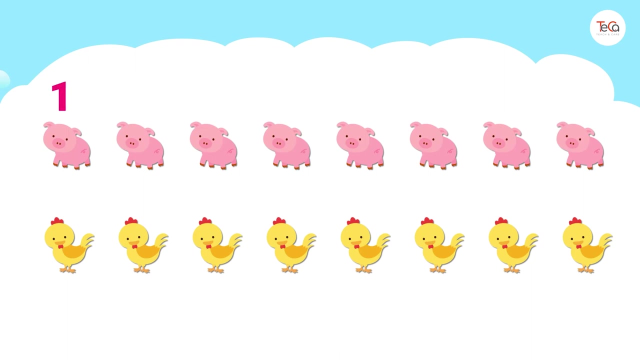 Now we have a number of pigs and chickens. The number of pigs is The number of chickens. Hmm, what do you think? Here we have 1,, 2,, 3,, 4,, 5,, 6,, 7,, 8 pigs. 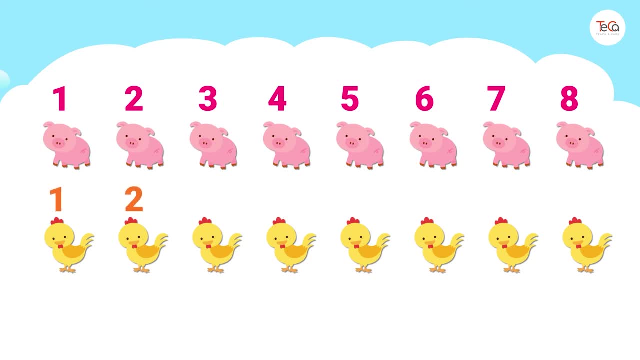 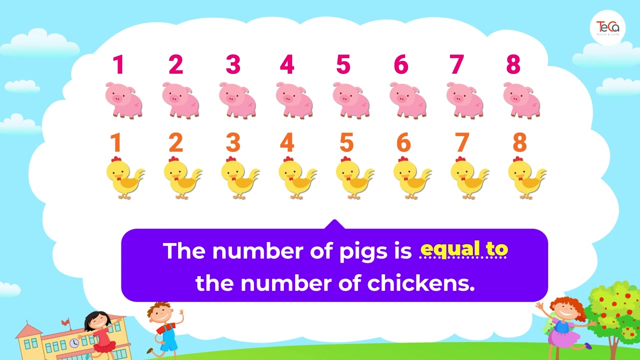 And 1,, 2,, 3,, 4,, 5,, 6,, 7, 8 pigs, 5, 6,, 7, 8 chickens. So the number of pigs is equal to the number of chickens.